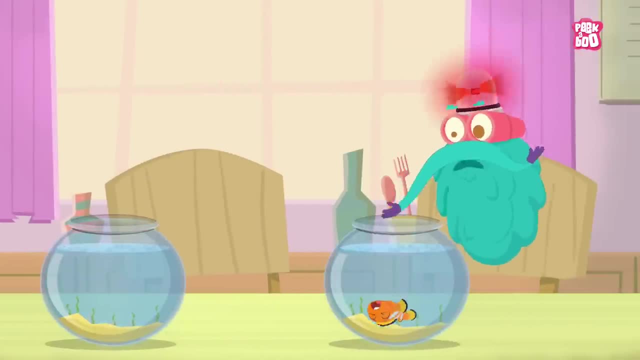 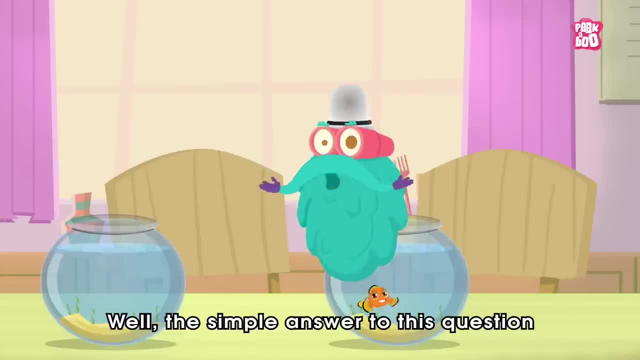 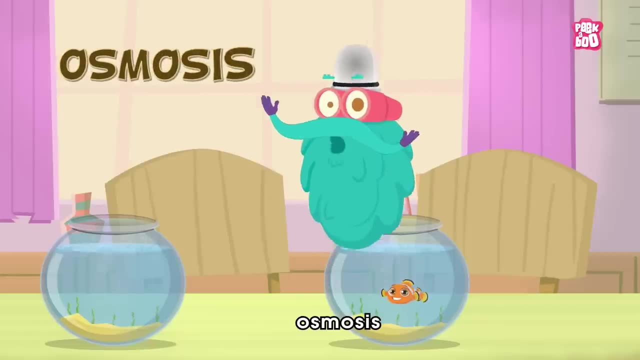 After all, it's water that too fresh. Well, the simple answer to this question is a fancy nancy word: osmosis. So in today's episode, In this episode, let us explore what osmosis is and how it works. 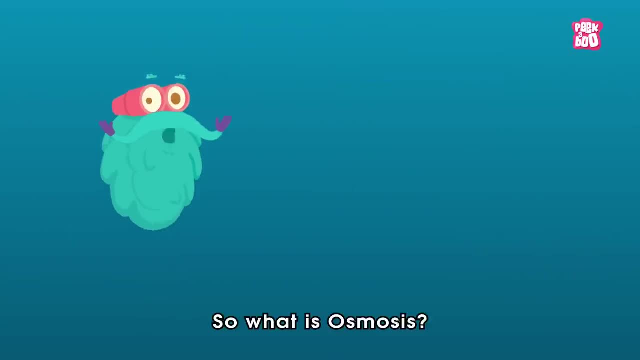 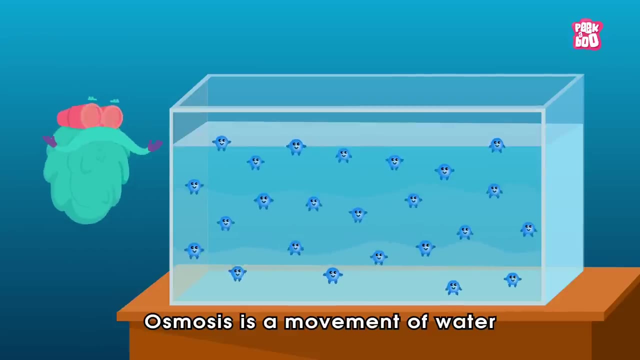 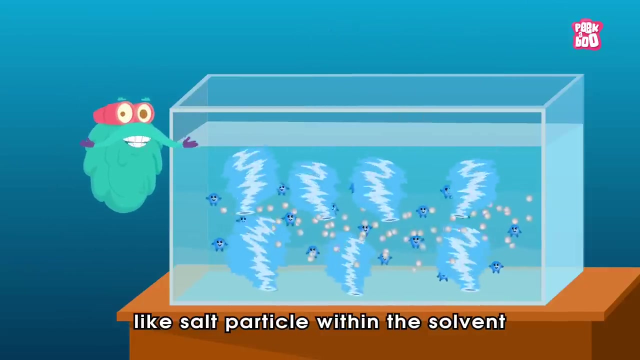 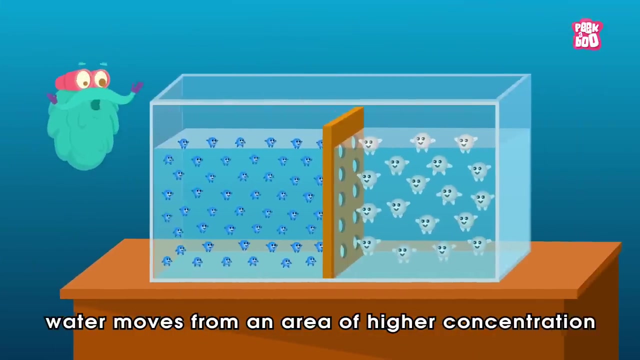 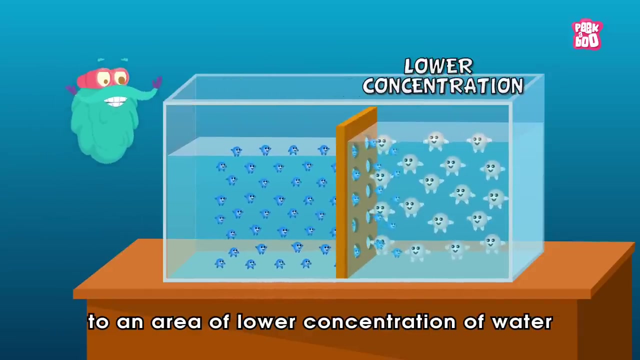 Zoom in. So what is osmosis? To keep it in simple words, osmosis is a movement of water, A special kind of mixture of solutes like salt, particles within the solvent, like water particle. In other words, during osmosis, water moves from an area of higher concentration to an area of lower concentration of water through a selectively permeable membrane. 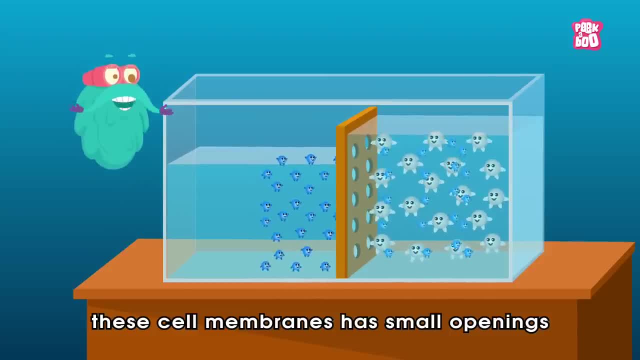 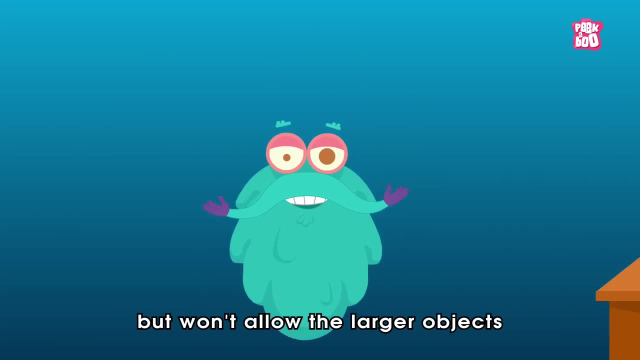 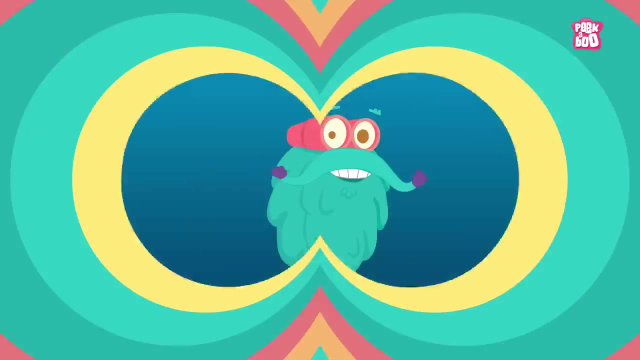 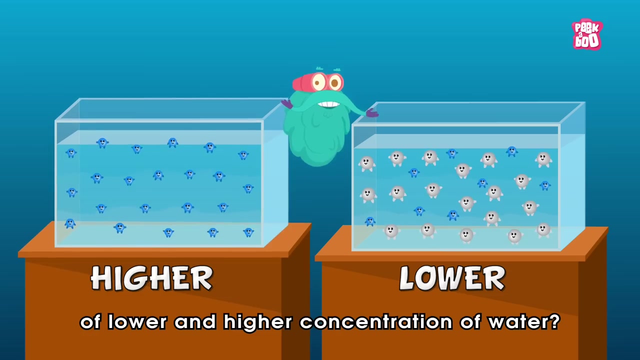 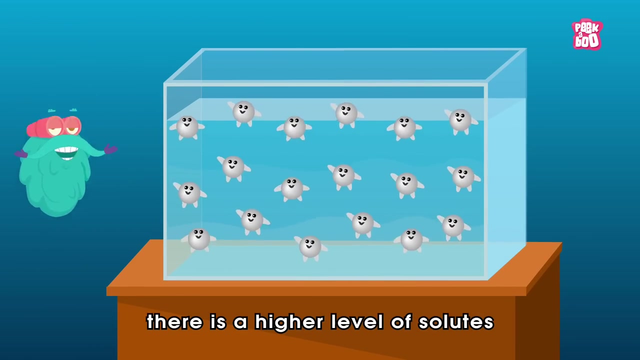 That is a cell membrane. These cell membranes have small openings that let the water molecules pass through it, But won't allow the larger objects, like salt molecules, to pass through it. But what is an area of lower and higher concentration of water? Well, it simply means that in a lower level of water there is a higher level of solutes like salt and sugar. 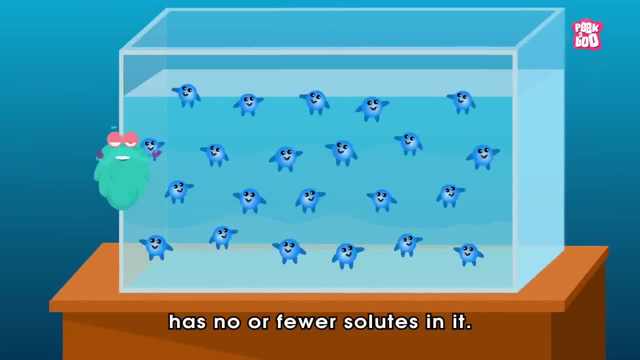 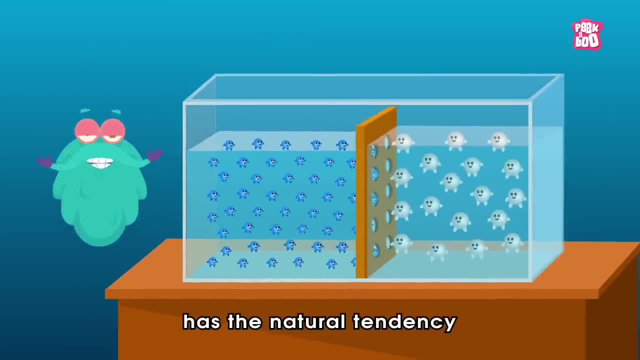 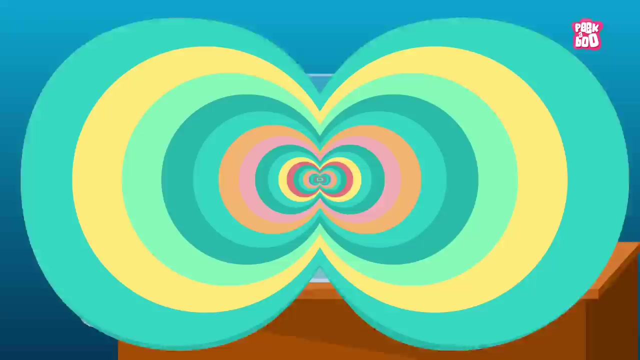 And the higher concentration area has no, or fewer, solutes in it. So all we need to remember is that the water has a natural tendency to move through the higher to the lower concentrated area. Let's try to understand it with an example. 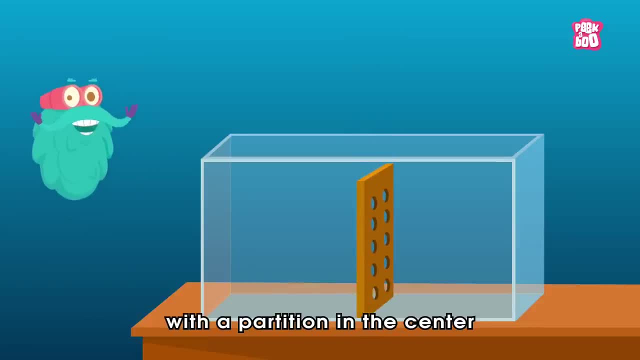 Imagine we have a glass tank with a partition in the center made of a semi-permeable membrane That can allow the solvents, like water, to pass through it, But not larger particles of solutes like salt. Now fill this tank with some fresh water on both the sides. 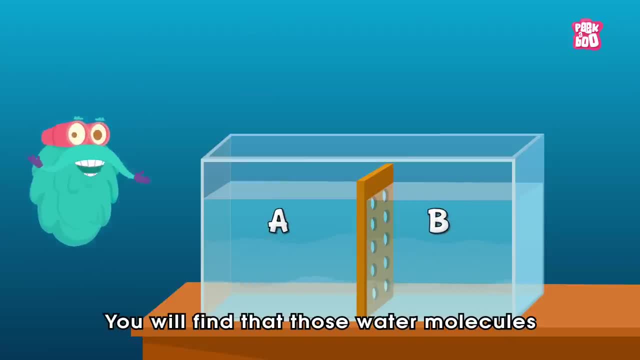 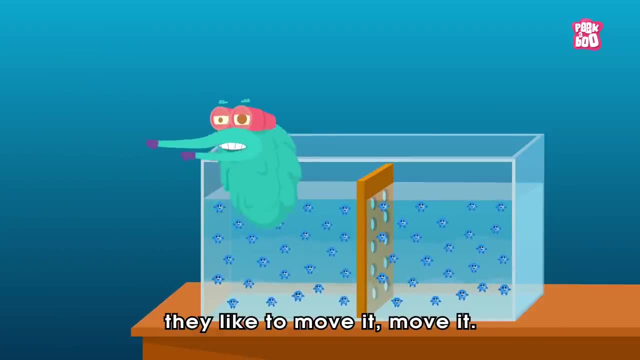 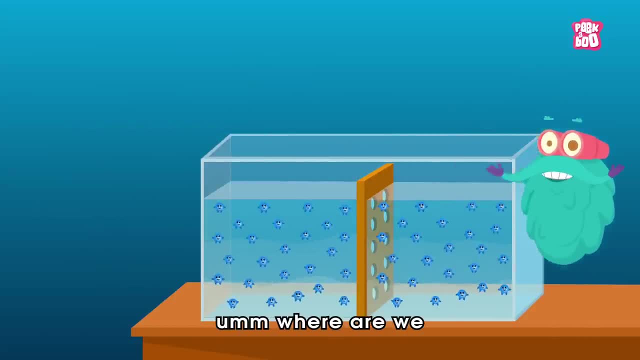 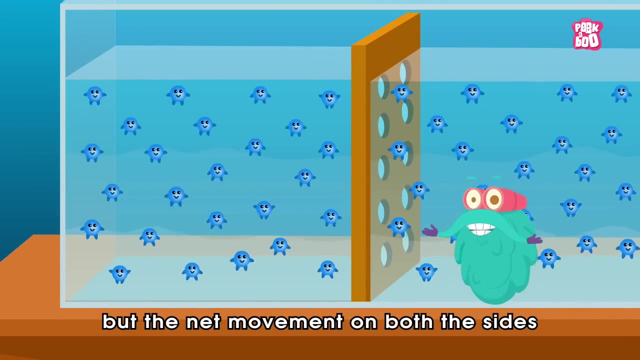 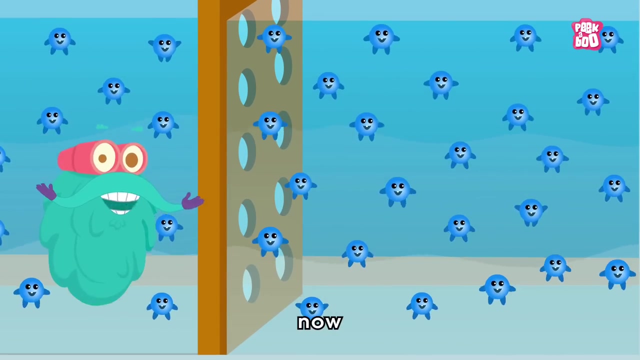 Sorry, I got carried away. Where are we? Yes, we can see these water molecules moving, But the net movement on both the sides are zero, Meaning the overall change in the direction of flow is zero. Now let's sprinkle some salt on side B. 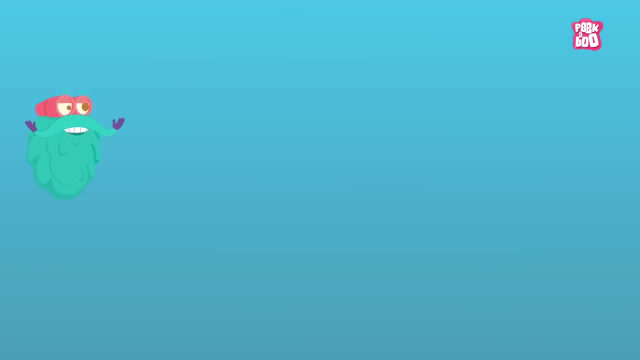 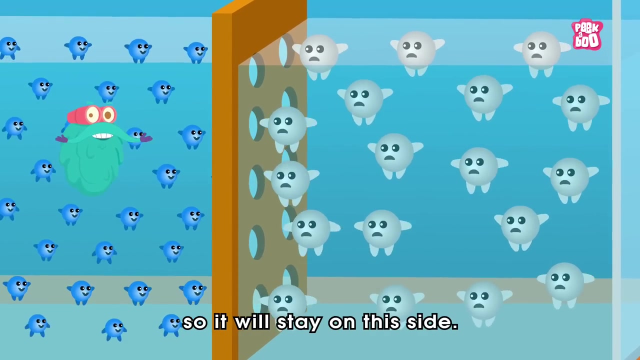 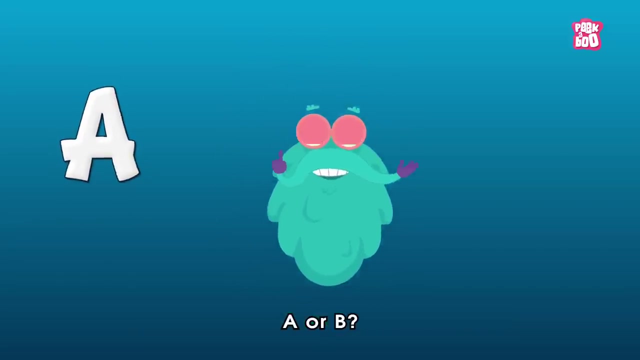 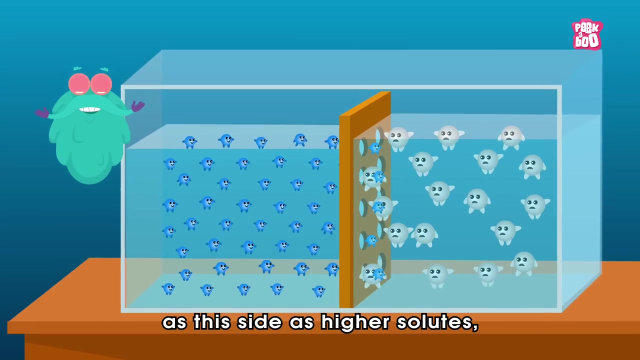 Some more, More Good Salt particles are too large to pass through this membrane, So it will stay on this side. So what do you think, friends, which direction the water will flow? A or B? Correct, It will move from side A to side B, as this side has higher solutes. 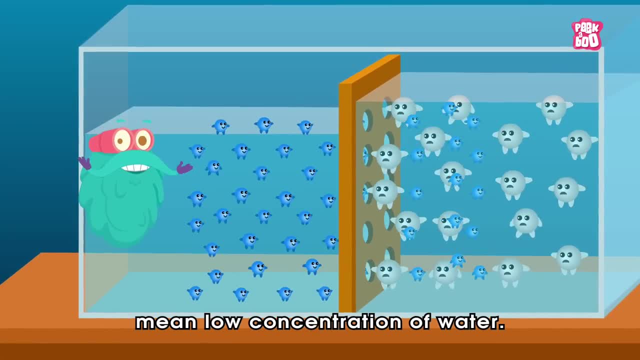 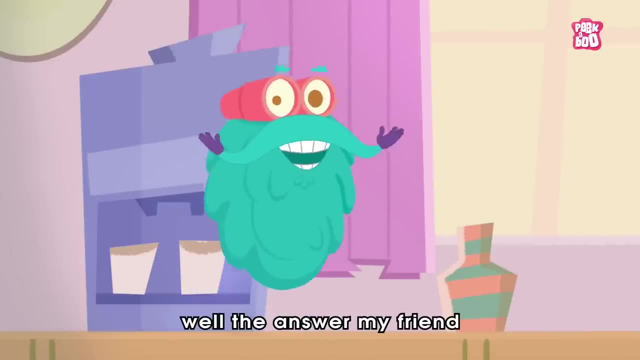 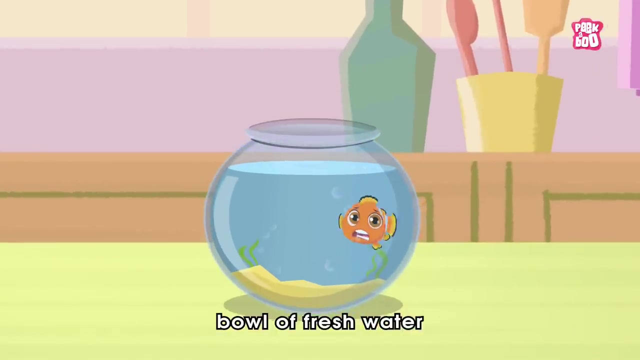 And higher solutes mean low concentration of water. So how does it affect our finned friend over here? Well, the answer: my friend is flowing in the water. Oh, it's an old song I love Again, sorry, Going back as you place the saltwater fish in a bowl of fresh water. there is a vast difference in high concentration level. 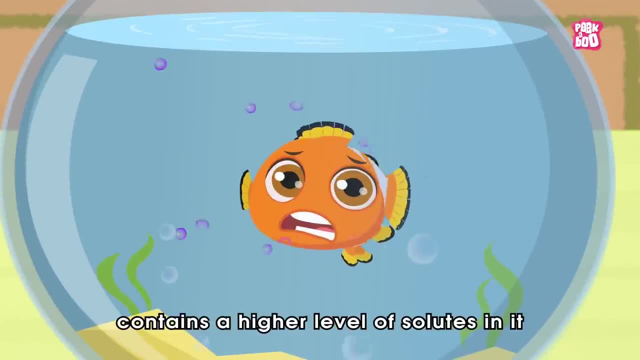 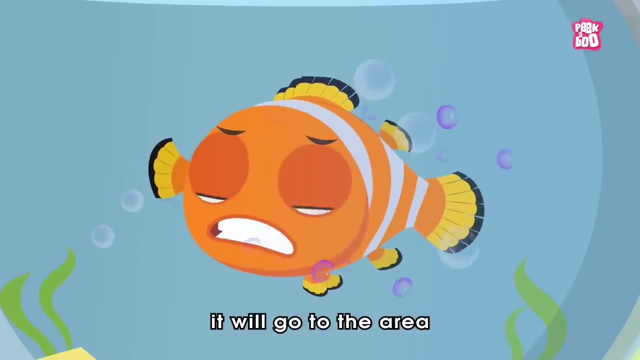 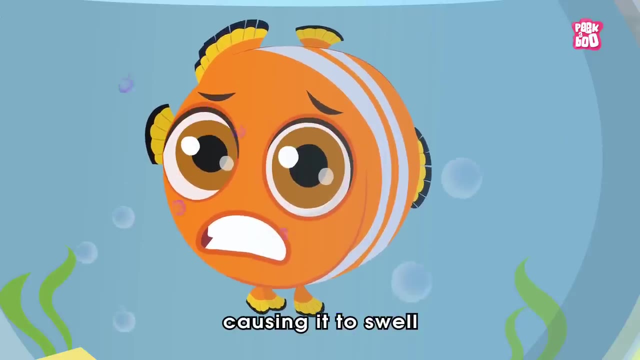 As the saltwater fish contains a higher level of solutes in it. So where will the water go? It will go to the area where there is a high level of solutes, and water will flow into the poor fish, causing it to swell.